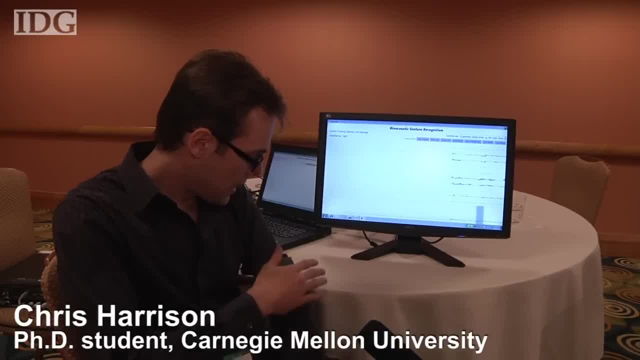 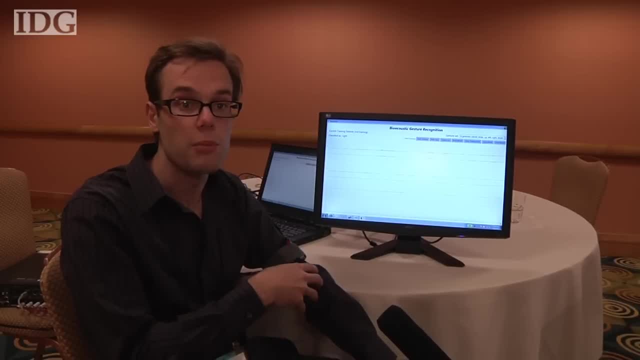 or cell phone. So Skinput works by having this armband with ten very specialized vibration sensors and it's basically acting like a microphone that's listening inside your body, And so when I do a tap, you'll see here that I get these very nice little ridges. These are actually 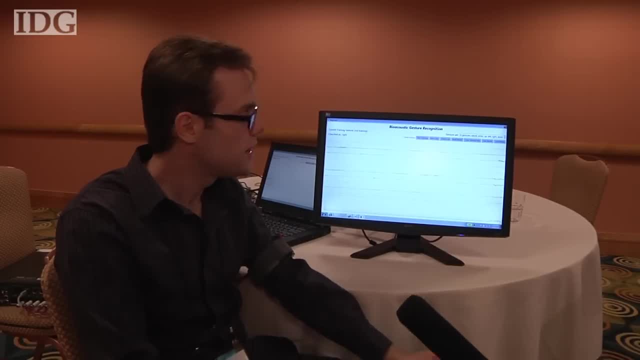 sensors from the ten. this is data from the ten sensors And it can actually listen to these effects, these kind of impacts traveling up through the bones and muscles and ligaments and so on, And it actually listens to what those sound like and it can classify them. 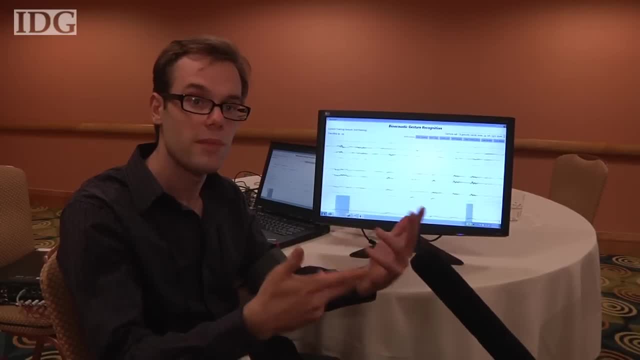 And if it learns what you know, for example, your middle finger sounds like, then it can say: oh, I just heard the middle finger, I just heard the pinky finger, I just heard your palm. And then you can bind interactive capabilities onto those. 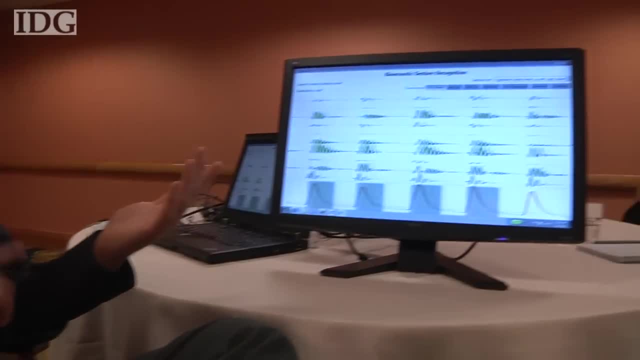 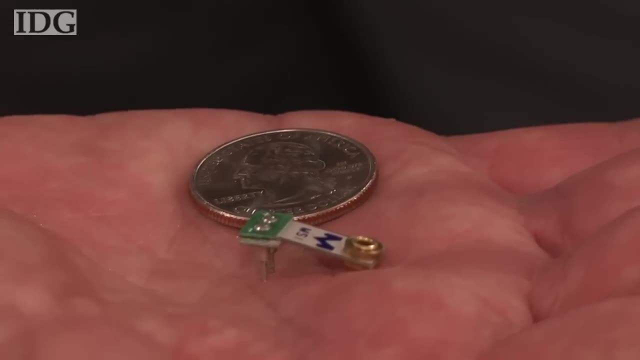 For each new user. it takes a minute or two to calibrate the system, and that's done by pairing an action with a tap on a certain part of the body. Ten of these small sensors in the armband collect the vibrations. The demonstration at the CHI conference used a. 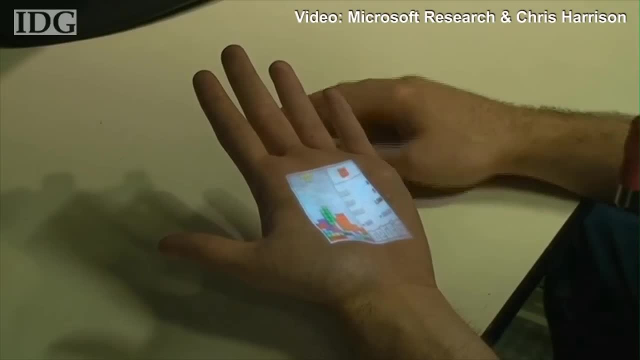 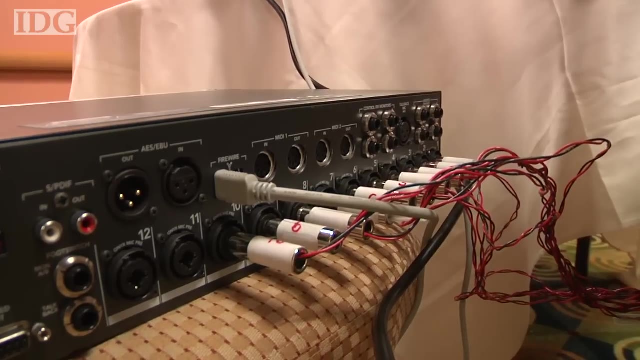 monitor to show the interface, but during another demonstration off-site, the team used a shoulder-mounted mini-projector to show the display on the body. The system now is quite bulky but Harrison hopes to scale it down. I think the main challenge, and certainly what we're going to be moving towards in our kind of immediate 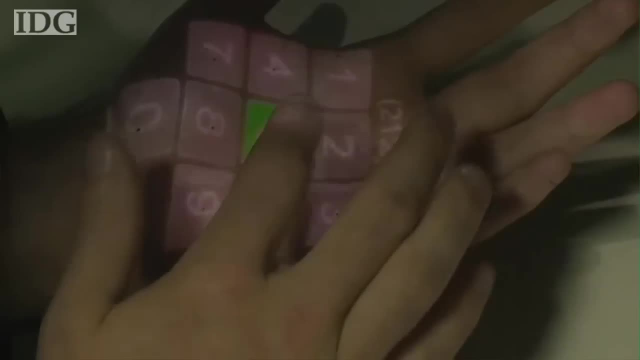 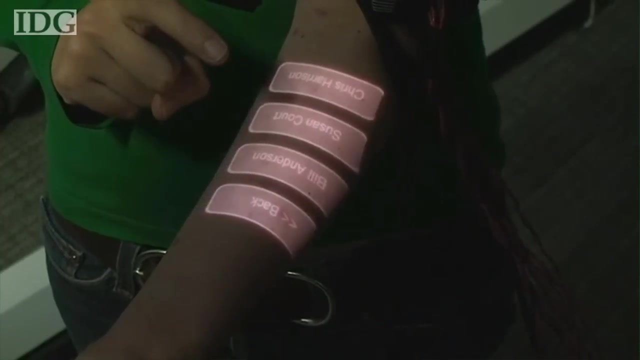 next step is shrinking the prototype down. So this armband is really quite large, but there's no reason why the sensors can't be very small, So maybe the size of a penny could encompass, you know, the entire armband that is now And that could really fit into the 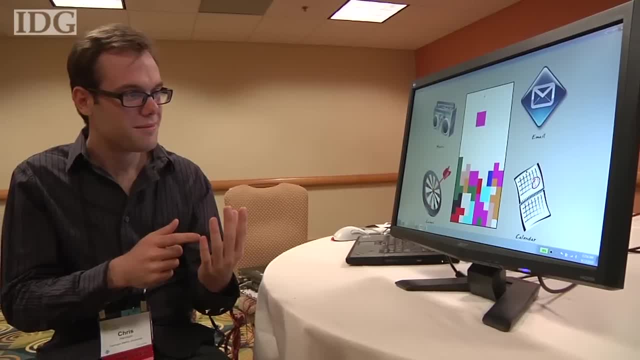 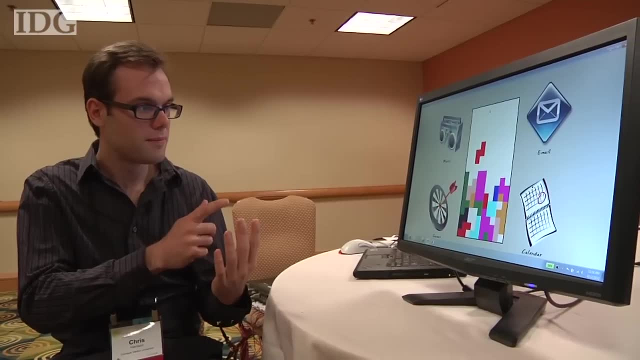 back of kind of your audio player that you might wear when you're out for a jog. Harrison, a PhD student at Carnegie Mellon University, said that in a lab test, jogging didn't interfere with the system. Right now the unit can recognize six assigned tasks up down, left, right, enter and cancel. 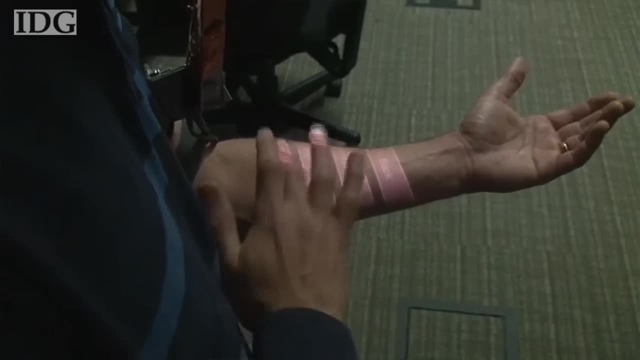 as more are added. the system needs to be more accurate. In kind of in the wild, and especially with like ten inputs, your accuracy is going to suffer like maybe 90, 95 percent accuracy, And that's not going to be acceptable. if people 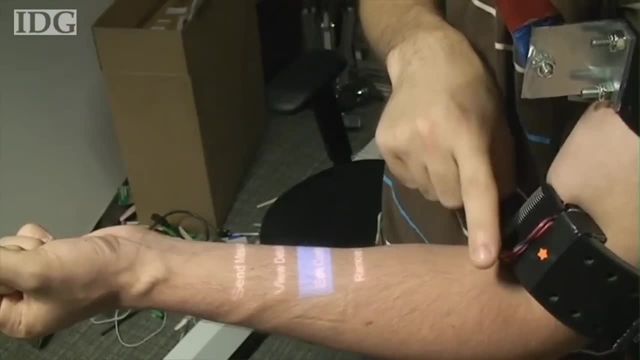 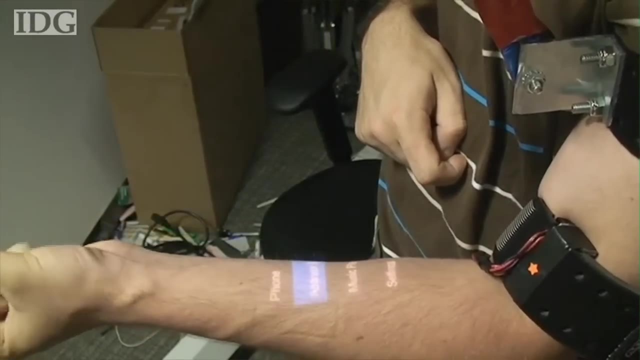 are going to want to do like text entry, And so we really need to push the accuracy up even better, into kind of the high 90s and maybe even to 100 percent for a lot of actions, if we really want this to be, you know, palatable for consumer electronics.